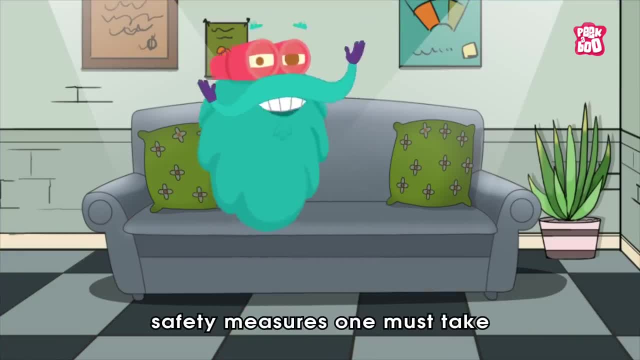 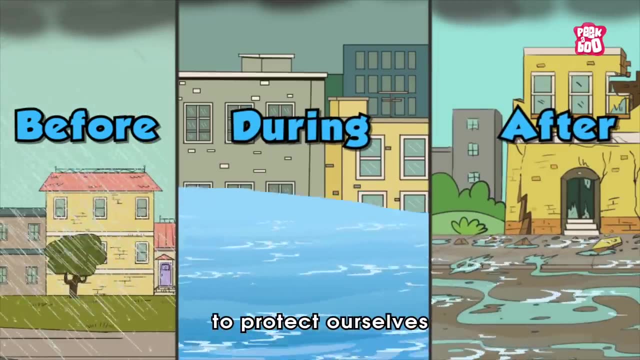 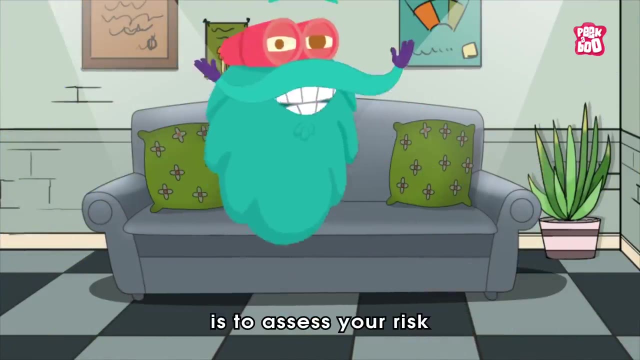 Therefore, we all must be aware of the safety measures one must take before, during and after the floods to protect ourselves and our loved ones. And the first step in flood survival is to assess your risk by listening to the weather report on the radio, TV or the internet. 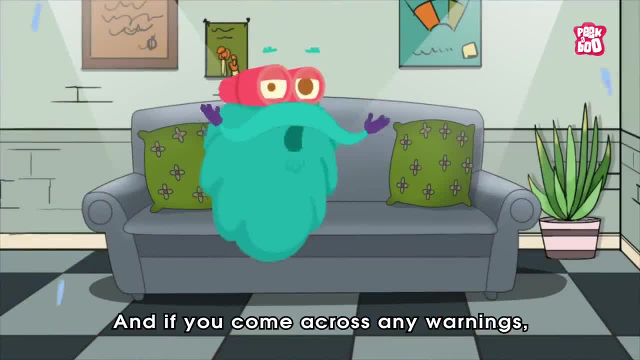 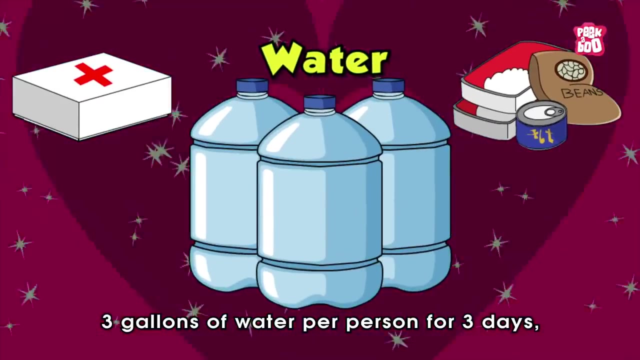 especially if you live in a coastal region. And if you come across any warnings, quickly share the news with your family. Then it is essential to stock up on first aid items, non-perishable foods, 3 gallons of water per person for 3 days, battery operated radio for weather reports. 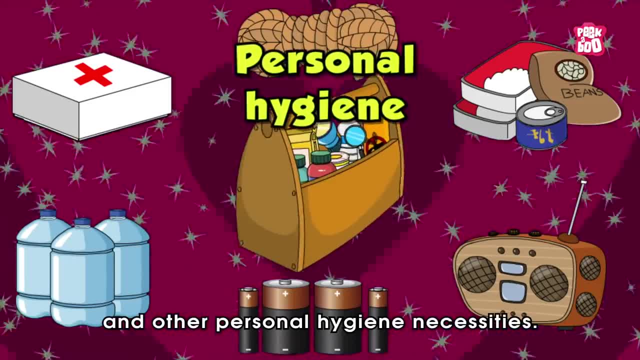 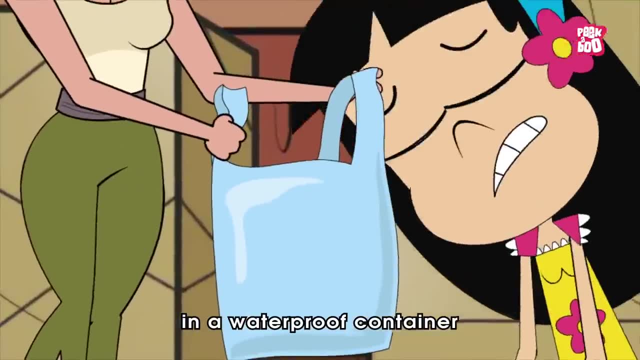 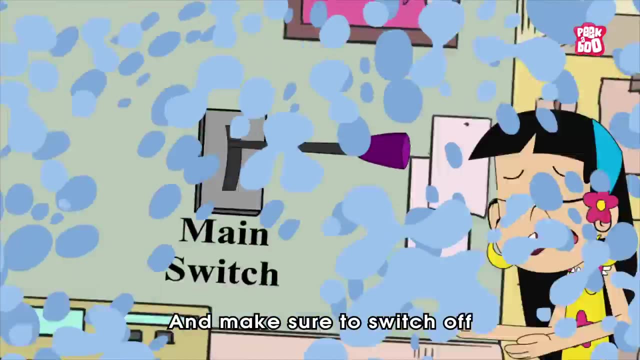 extra batteries, a rope and other personal hygiene necessities. Also, make sure to keep important documents in a waterproof container And, if possible, move valuables to a safe place, And make sure to switch off electrical appliances, as it can cause electrical fires. 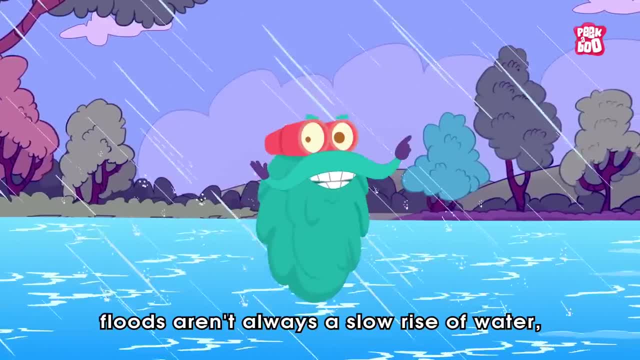 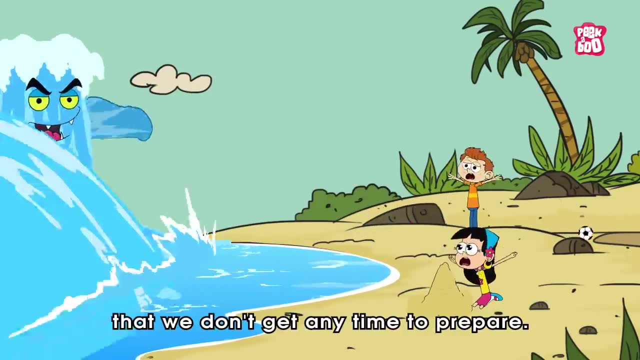 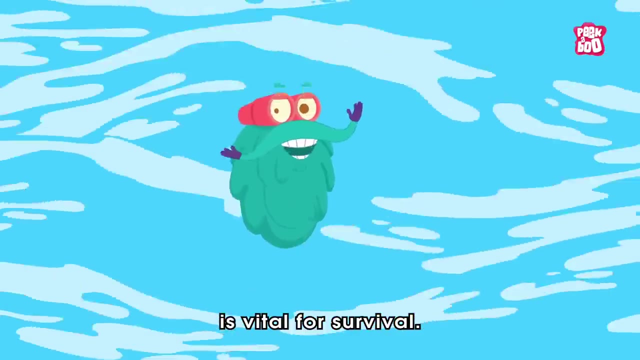 But here is a thing, my friends: floods aren't always a slow rise of water, And at times it can happen so quickly that we don't get any time to prepare, And that's why what you do during a flood is vital for survival. 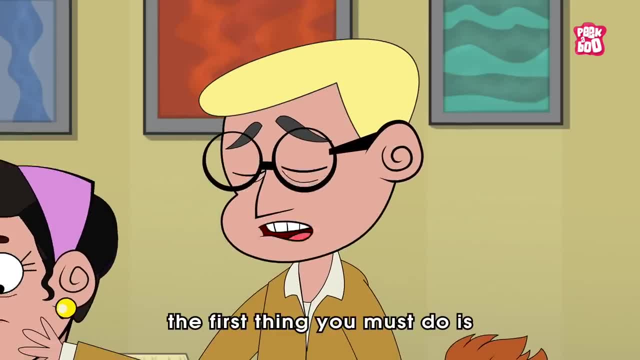 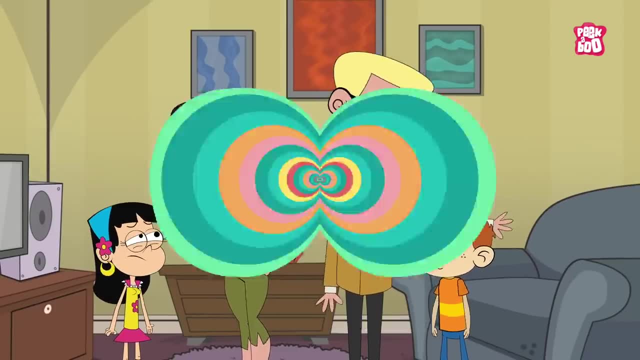 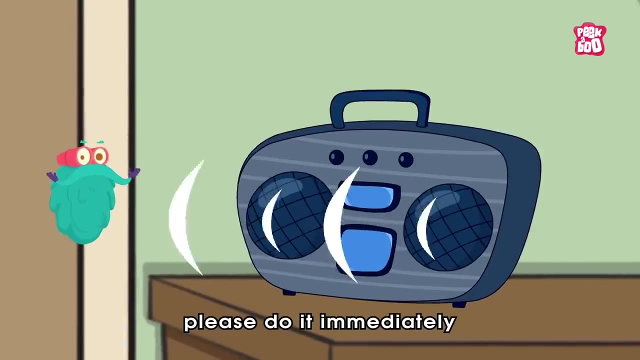 For that reason, the first thing you must do is always listen to adults and stick with your family no matter what. And, most importantly, if your local authorities ask you to evacuate, please do it immediately and go to the top floor terrace or roof of your house. 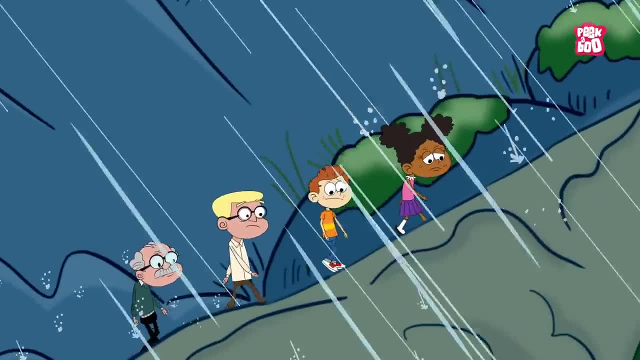 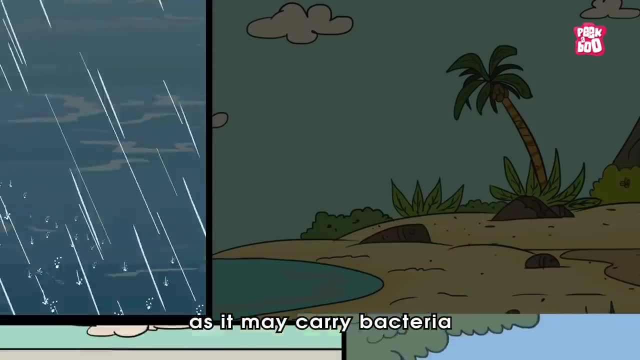 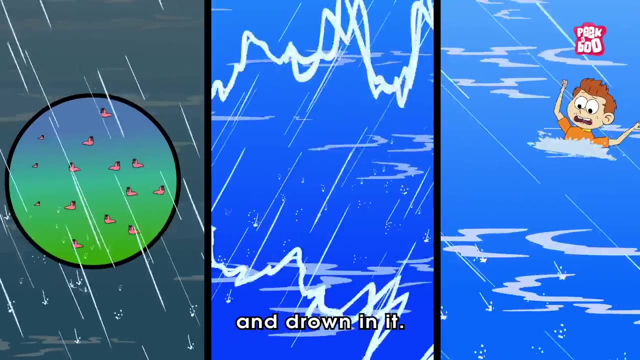 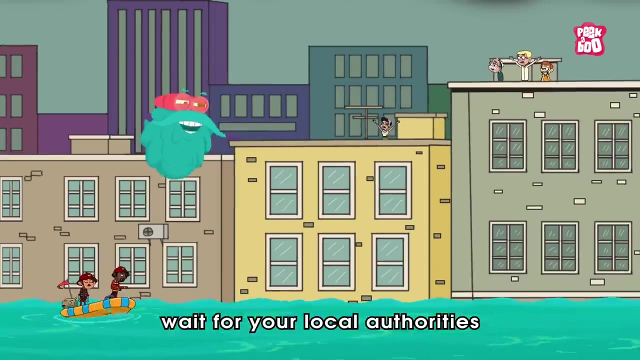 Or, if possible, move out to the higher ground, But make sure to avoid getting into dirty water or jumping into it, as it may carry bacteria or can be vulnerable to electric shock or worse, one can get dragged away and drown in it. And once you see the water level going down, wait for your local authorities to examine the place.